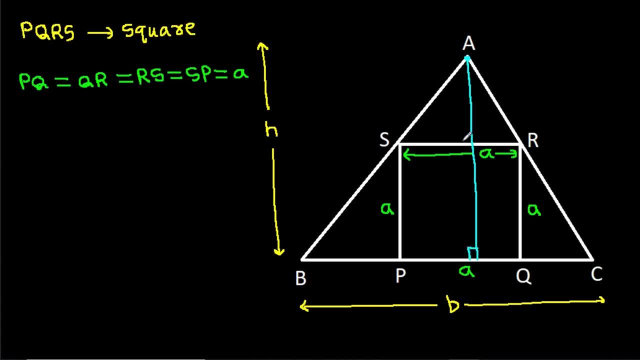 on BC. suppose this point is M and this point is N, Then MN. it will be equal to SP, that will be A And AN. it is height of the triangle, that is H, So AM it will be equal to AN minus MN. 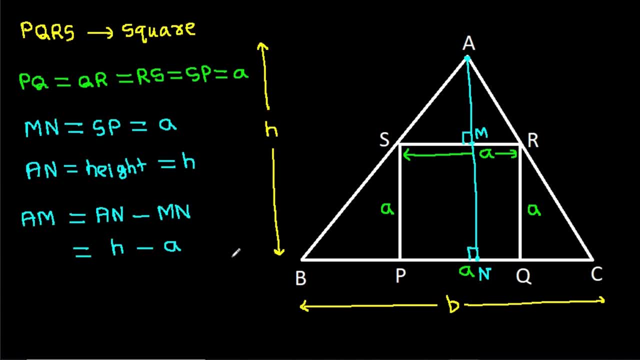 That will be equal to H minus A, AM it will be H minus A, And now PQRS it is a square, So SR it will be parallel to PQ. That means SR it will be parallel to BC. 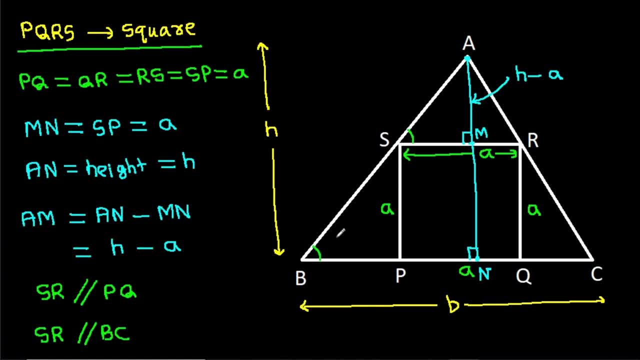 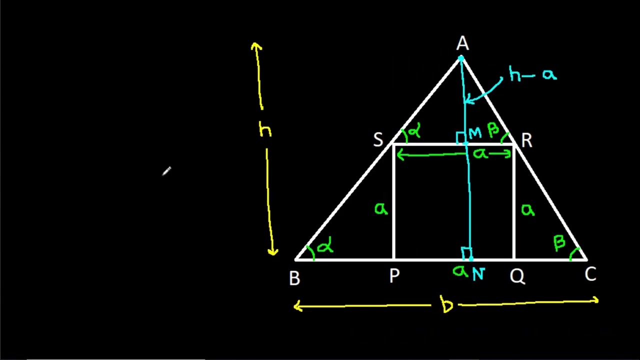 That means these two angles they will be equal And these two angles they will be equal. And Now in triangle ASR and triangle ABC we have: angle ASR is equal to angle ABC and angle ARS is equal to angle ACB. 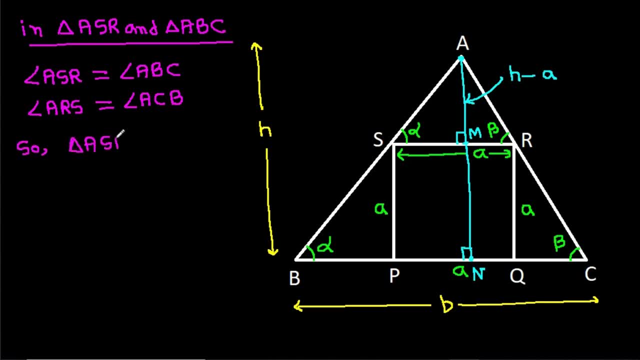 So triangle ASR, it will be similar to triangle ABC. Hence ratio of base: SR by BC it will be equal to ratio of height AM by AN. And SR is A by BC is B, It is equal to AM is H minus A.